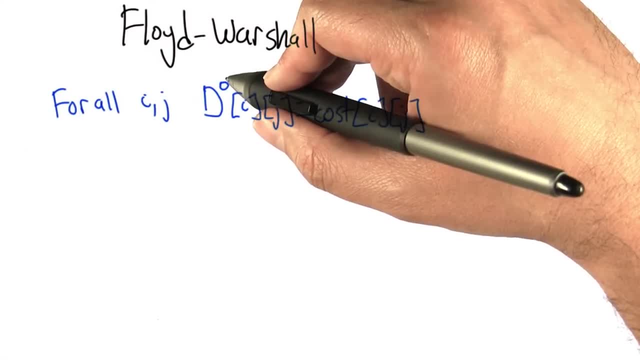 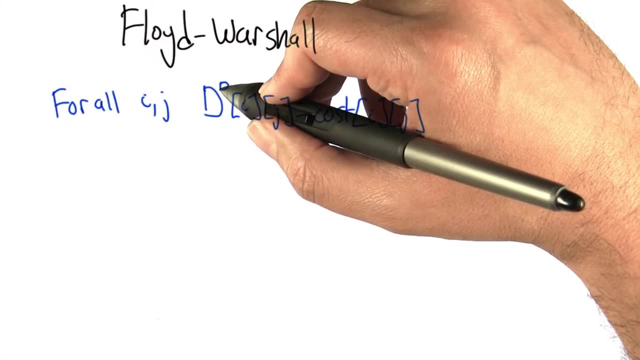 So we can initialize d0.. So this is the length of the shortest path from i to j using nodes only numbered less than 0, which is to say no intermediate nodes. That's just the direct cost of going from i to j, So we could just fill in from the cost in our graph. 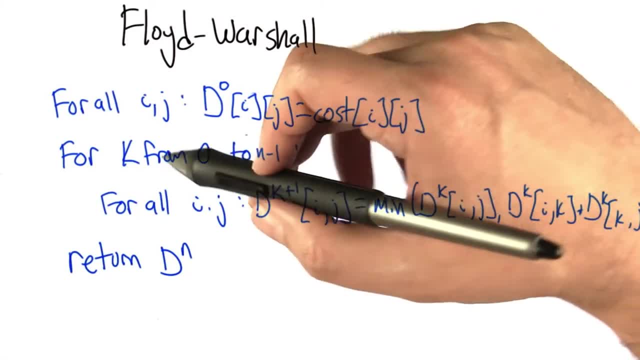 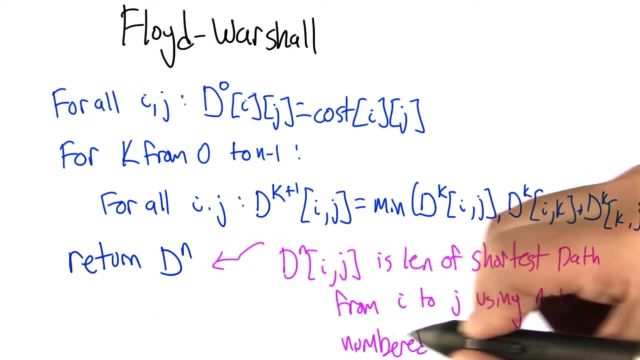 We can fill in this matrix And once we have d0 initialized, we can run k from 0 to n-1.. And for each pair of i and j we take dk plus 1 to be the smaller of dkij and dkik and dkij added together. 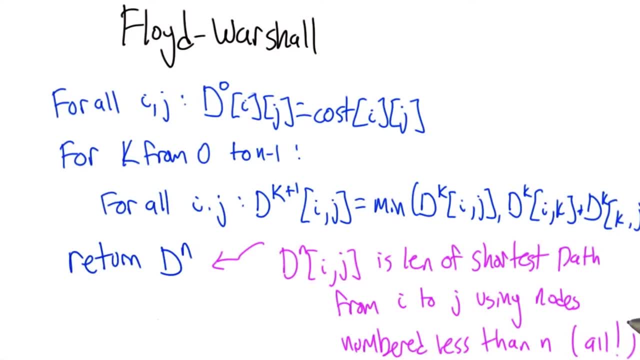 just as I was just describing before. When this is all over, when this loop is done, we have dn. Well, dn, but dnij is the length of the shortest path from i to j, only hopping on nodes that are numbered less than n, but that's all the nodes. 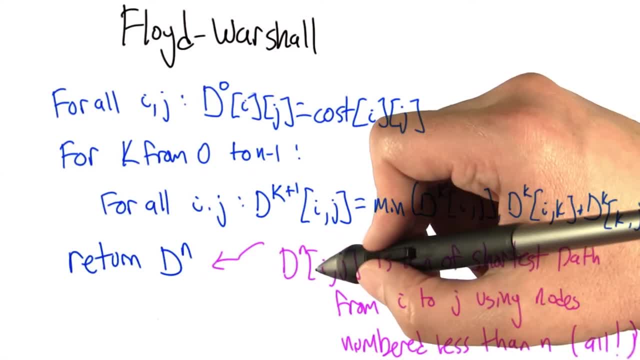 All the nodes are numbered less than n. They're all numbered from 0 to n-1.. So this is the length of the shortest path from i to j. It's restricted full stop. So that's pretty cool. And if you think about what's going on here, 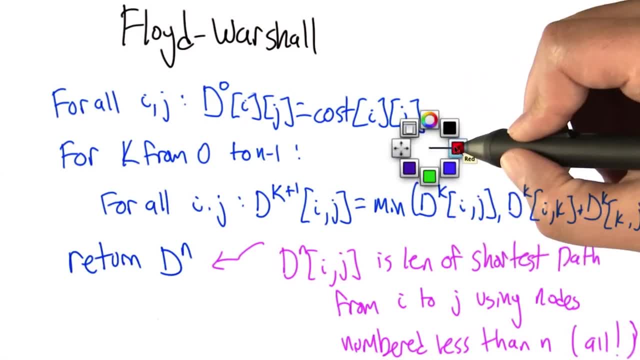 this initialization step runs over all pairs of nodes, So that's n squared. This loop runs over all pairs of nodes, n squared, but it does this for each value from 0 to n-1.. So altogether we're talking about n times n squared, or n cubed. 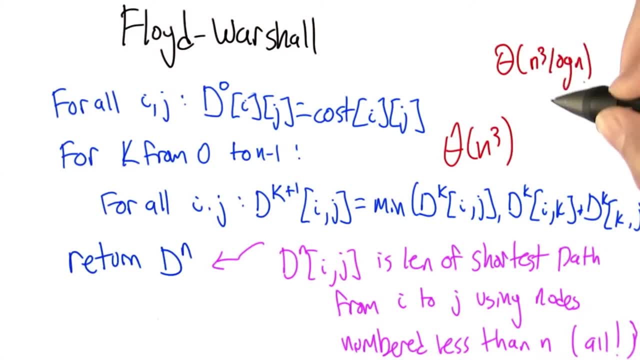 This is better than the n cubed log n we get by applying repeated Dijkstra to a dense graph. So for a dense graph you're better off using Floyd-Warshaw n-cubed instead of the n cubed log n. 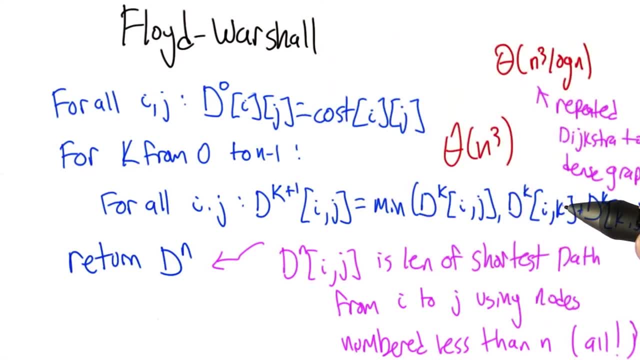 Now, log n is often not that huge a number, so your mileage may vary. You should actually try the overhead, But boy, it's hard to imagine having less overhead than this. It very straightforwardly runs through the n cubed possibilities And in fact, if you do this carefully, 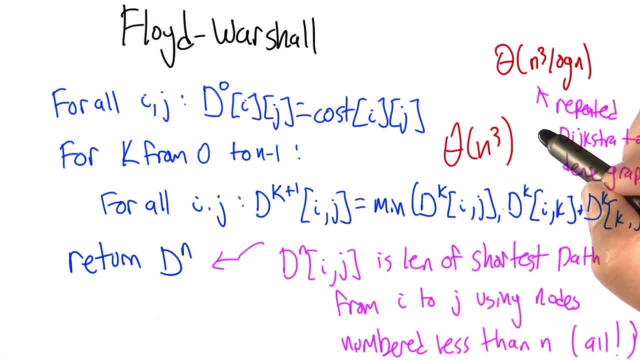 you don't need to keep a separate D matrix for each of these cases. You can actually do these updates completely in place, So the storage is pretty low too.